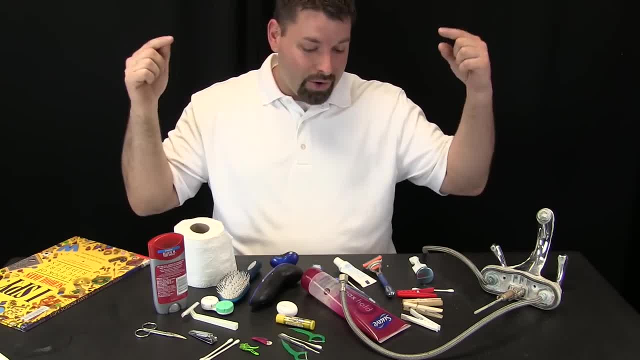 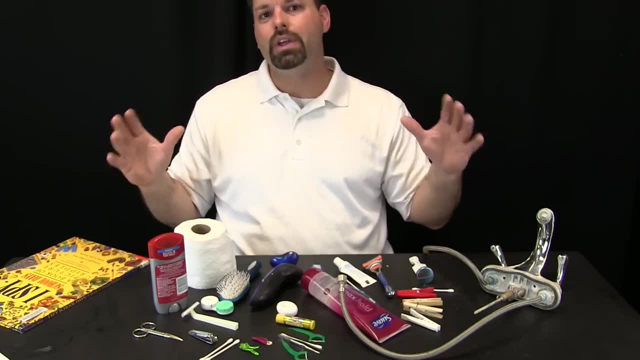 actually all about the simple machine science that are found in these items in my bathroom. Now, remember, simple machines are anything that makes our work easier. So I am going to read the first line of the poem and then we are going to go on a little hunt to see if we can find the thing. 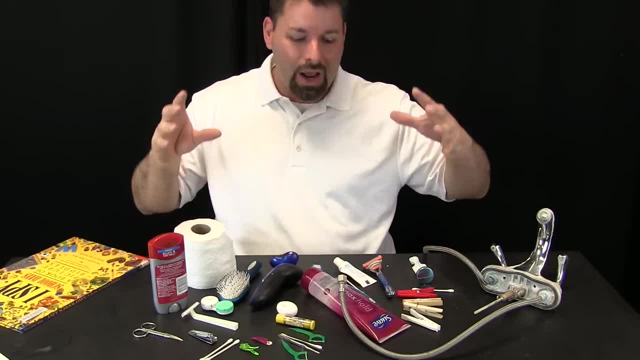 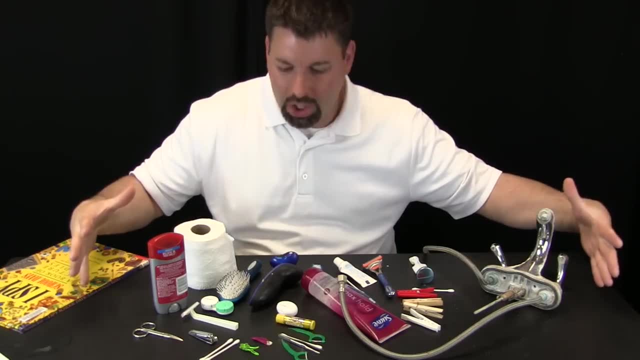 that the poem is talking about. But we are not just going to see if we can find it, we are going to try that thing out to see if it really does match the clue from the poem. So take a look at what kind of things we have in front of us. So we have zoomed in so you can take a closer look at. 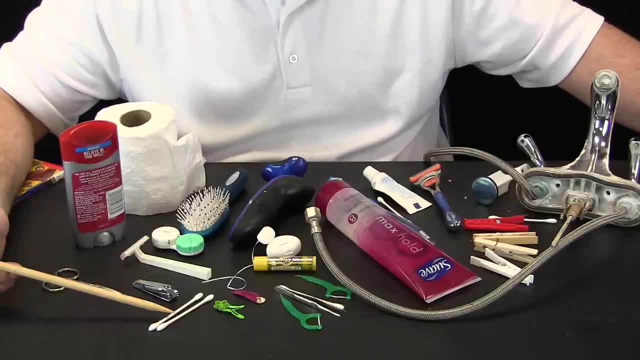 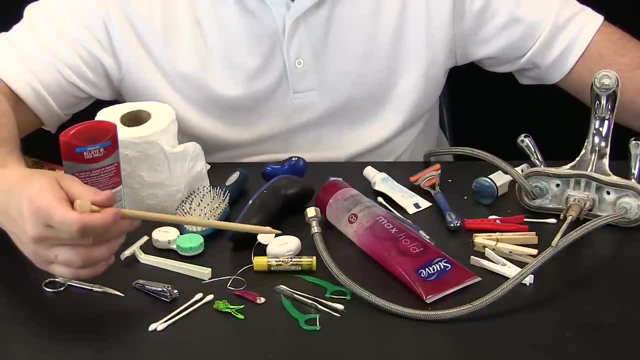 some of the items We have: scissors, fingernail clipper, Q-tip hair beret tweezers. that is a flossing stick. Here is a tub of floss. We have chapstick, hair gel, deodorant, a brush container for my contacts. 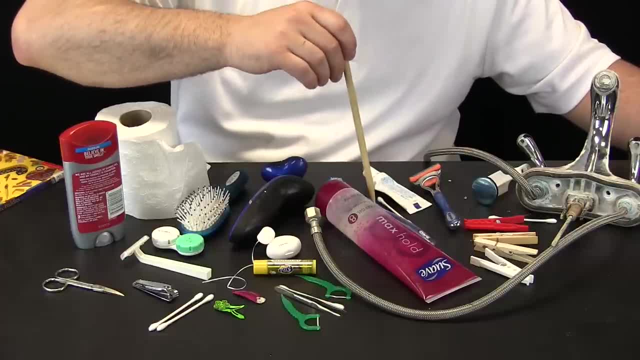 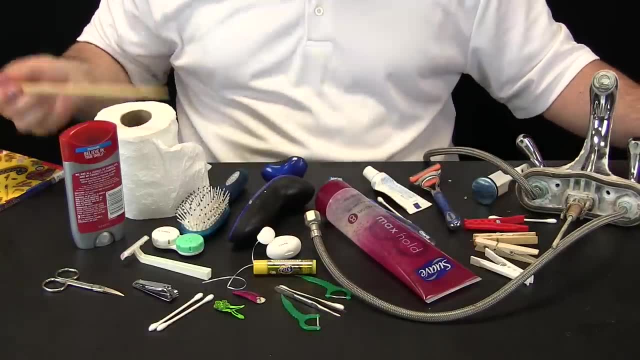 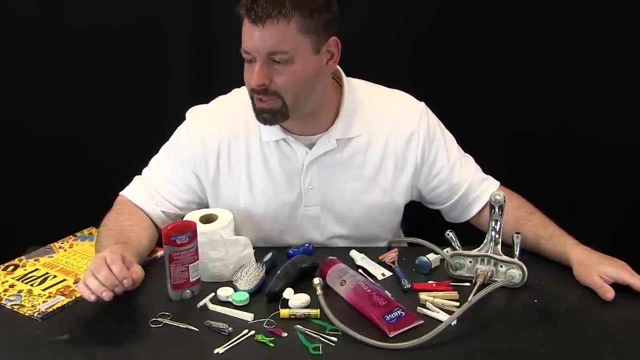 a razor, an electric razor, a toothbrush, a tube of toothpaste, some clothes pins, This right here is a faucet on my bathroom sink and we have a roll of toilet paper. So here is the first line of the poem, and it actually has two clues. So here we go. I try a lever that stops the drain. 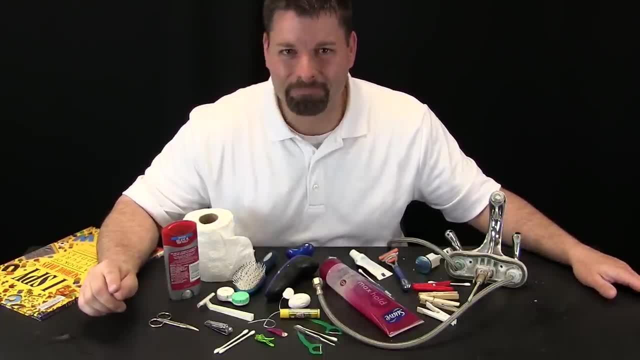 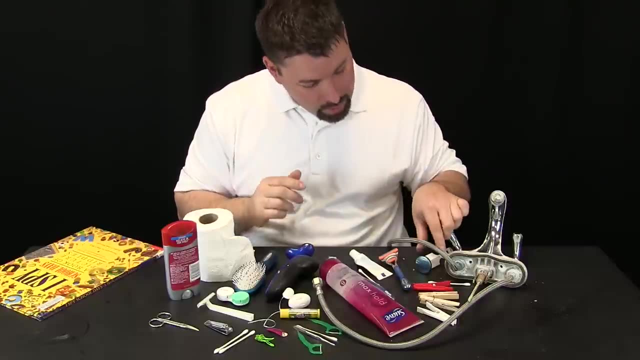 and a cap that works because of an incline plane Stopping a drain. Well, remember, what do you think? Look around, What is going to stop a drain? I look at this thing and this looks like it fits into the sink. Now I could not bring in my whole. 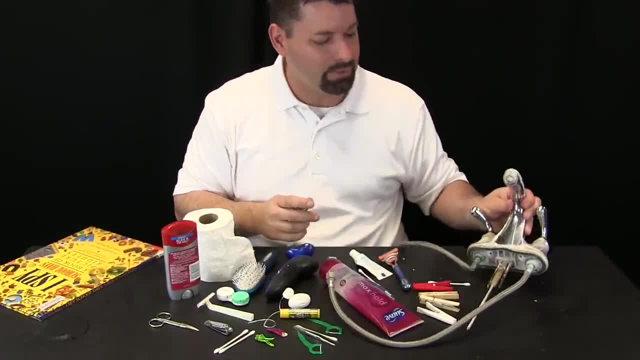 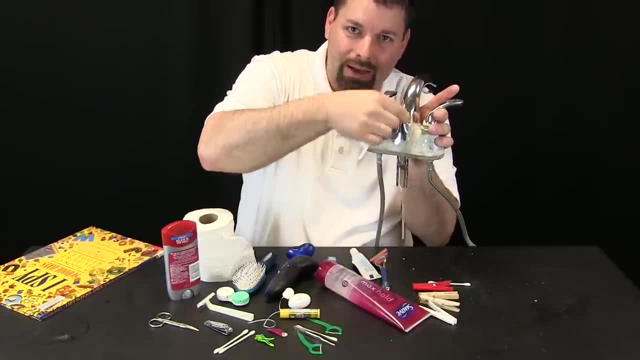 bathroom sink, but I could bring in the faucet, And here is a faucet. I am going to spin the faucet around and most sinks. you will be able to see this little thing in the back When I lift it up. what does it do? Well, this is my sink stopper and it sits in my sink. and when I pull, 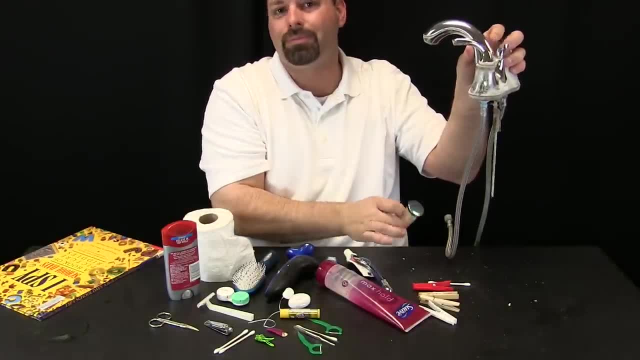 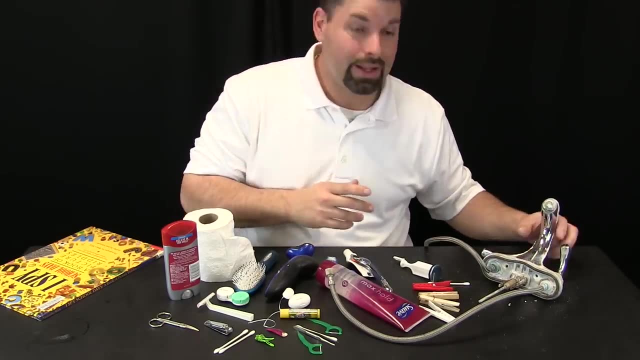 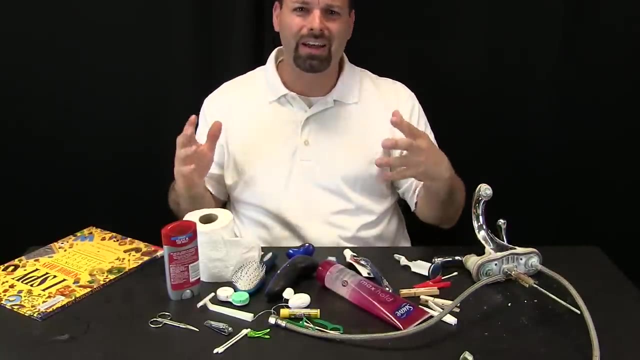 it down. guess what happens: The sink stopper goes down. I think we have found the thing that stops a drain. Now, what about? and it is not just a thing, it is a lever that stops the drain. What about a cap that works because of an incline plane? Well, what is an? 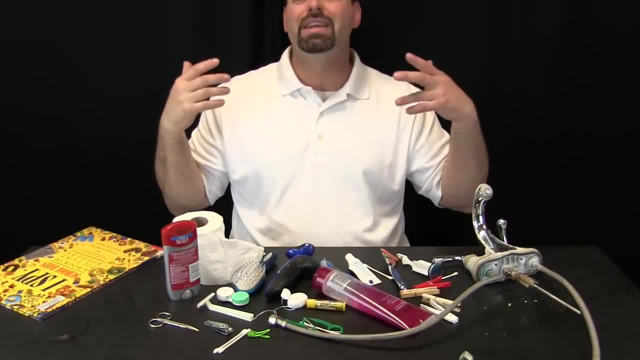 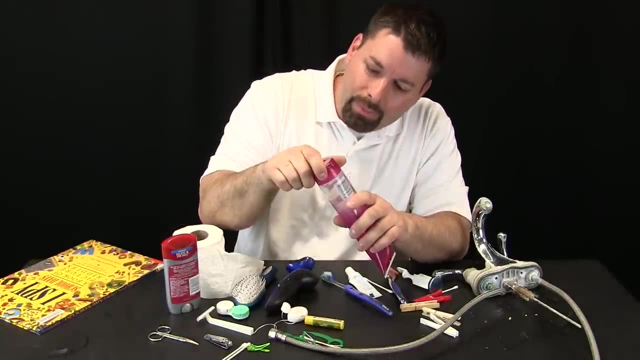 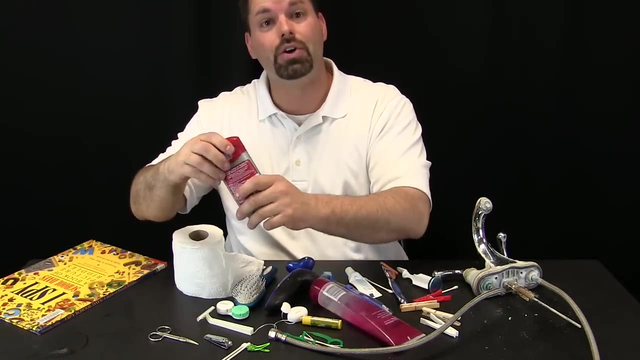 incline plane. So now we are on to our cap that works because of an incline plane. Let us look at some caps and try them out. So I have a cap to some hair gel. How does this cap work? Well, it flips open and that does not look like an incline plane to me. What about my deodorant? 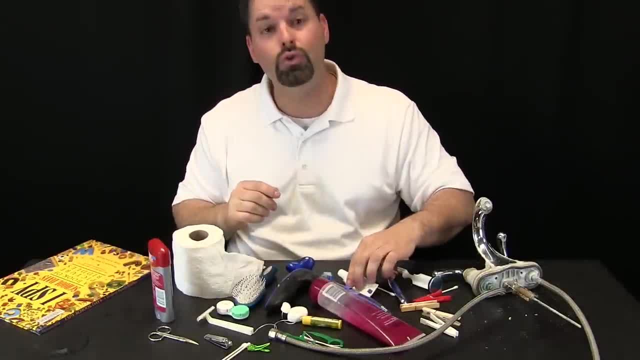 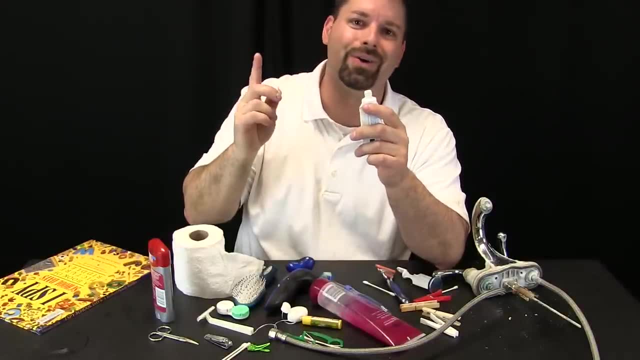 Nope, no incline plane there. Let us try toothpaste. Here we go. I do not have to, I cannot pull it, I have to unscrew it and what do you know? By trying it out, I think we have found our incline plane. If you look carefully, we are going to zoom in. 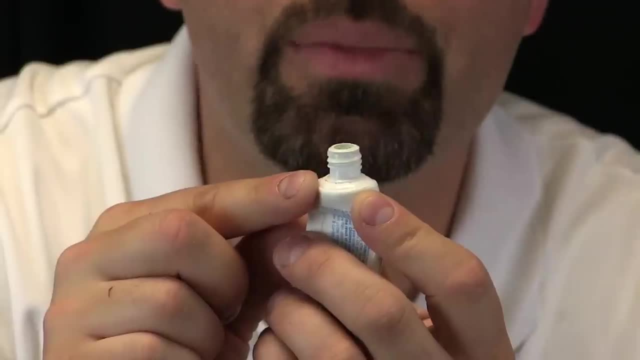 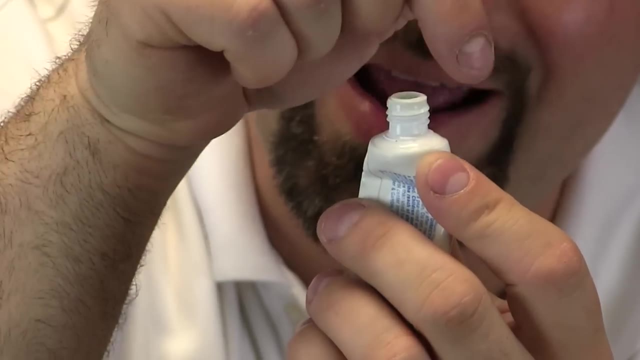 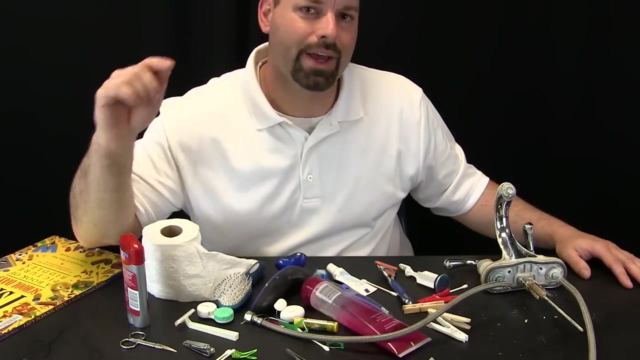 so you can see it. Take a closer look at the cap. Take a look at the top of this tube of toothpaste. I can see an incline plane that is slanted, but that incline plane is wrapped around the top of the tube. I found a cap that works because of an incline plane. Here is the next line of the poem. 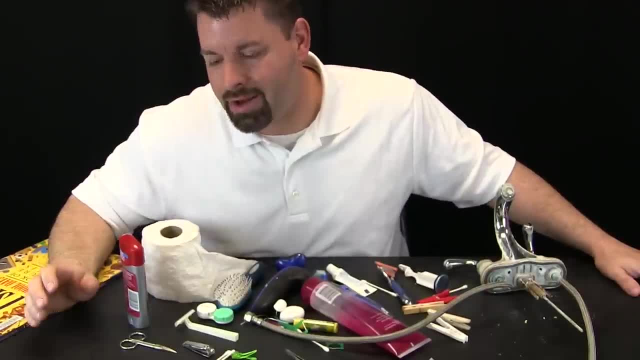 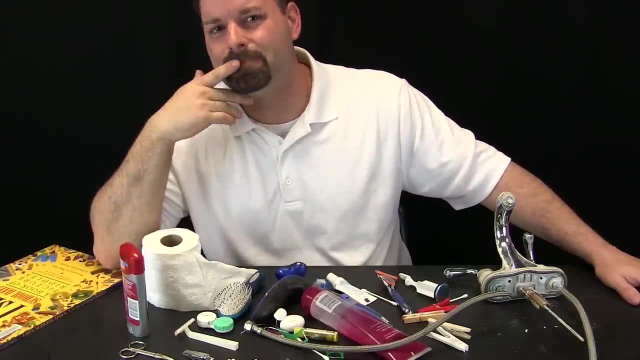 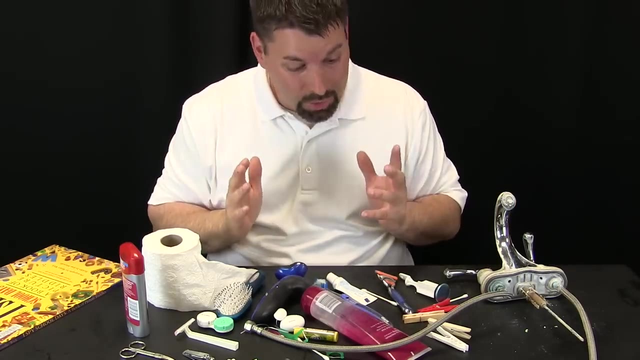 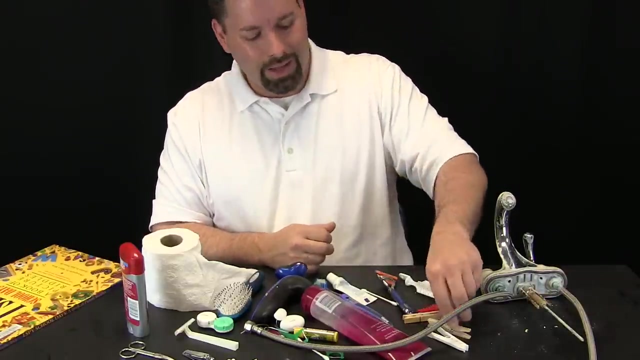 with our next two clues. I try a lever that pinches and grips and a wedge that separates cuts and clips. So let us start with the first one. I try a lever that pinches and grips. What could pinch and grip? Well, I see two things. Do you see them? Let us try it out. Let us try this. 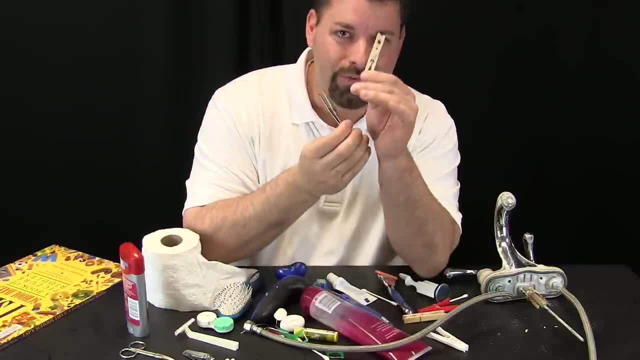 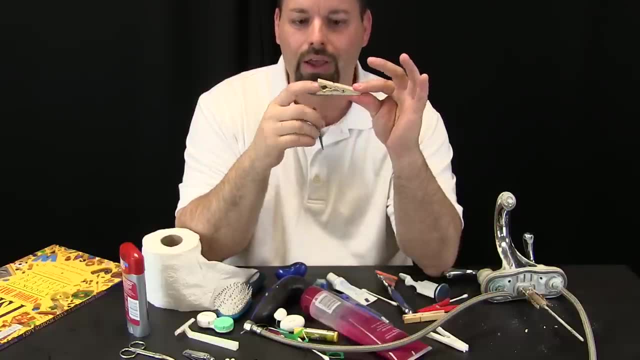 and let us try this. What are they? Well, I have a clothespin and I have a tweezers. Let us see if it actually pinches and grips. So here is my lever. You can see it work and it does pinch and grip. I 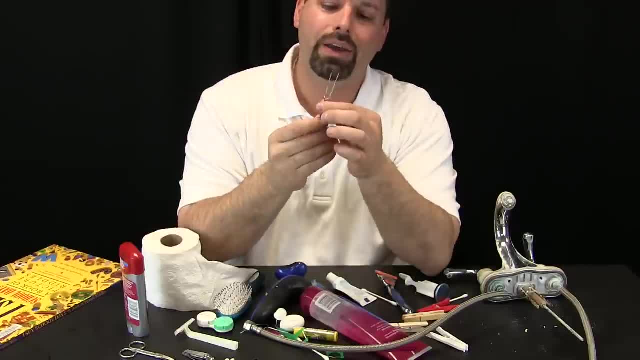 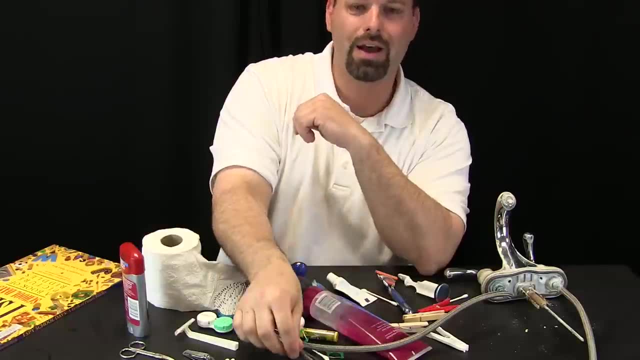 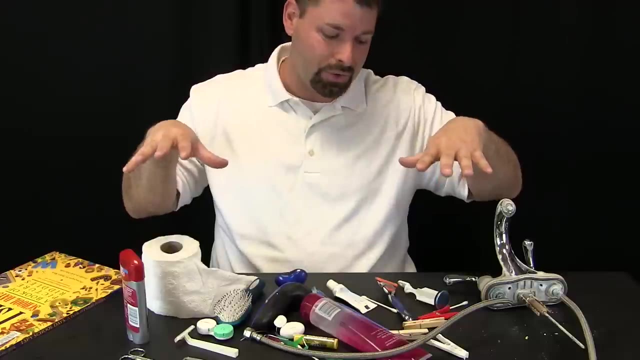 can use this to hang clothes out on the laundry line, or I could use my tweezers, and this does pinch and grip. I think we found it just by trying it out. Now we are looking for a wedge that separates cuts and clips. So what things here do you think we could try that actually cut? 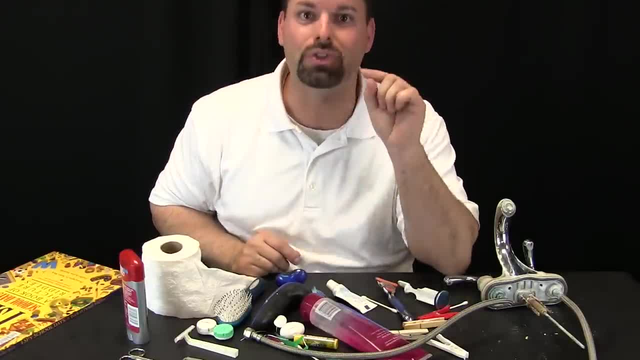 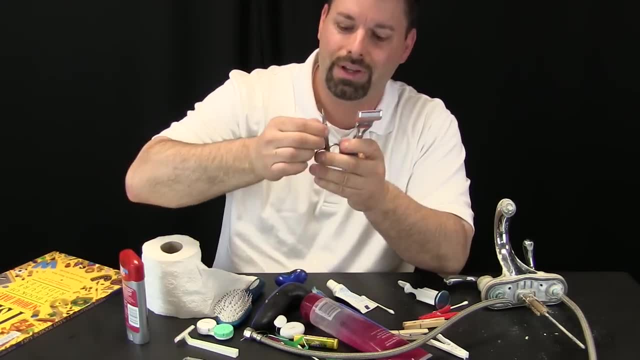 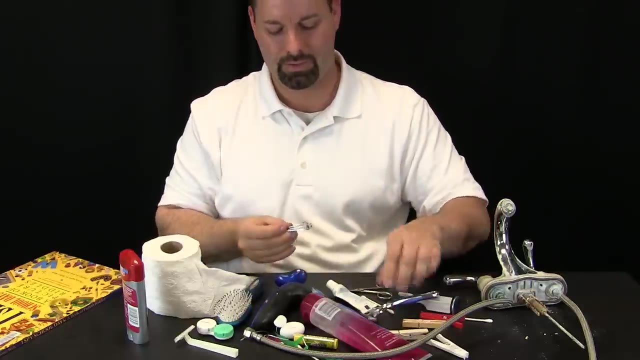 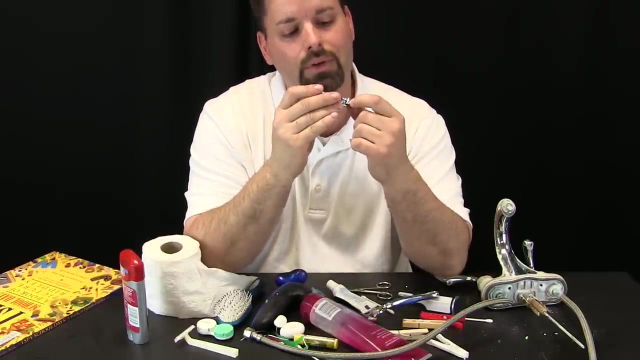 clip and separate. I see a couple of them. Do you see them? I am thinking a razor, a scissors and this a fingernail clipper. Why do not we try them out? Wow, it almost looks like. well, I will try it out on my fingernail. Line it up, clip it. 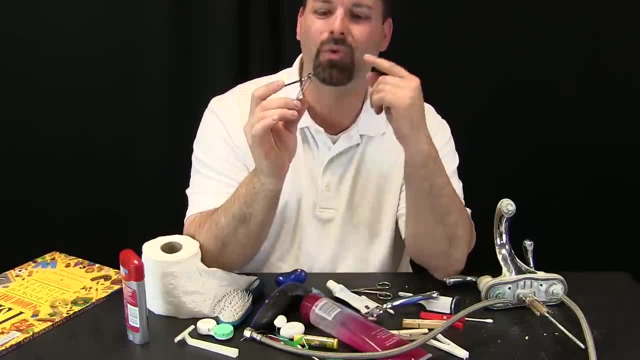 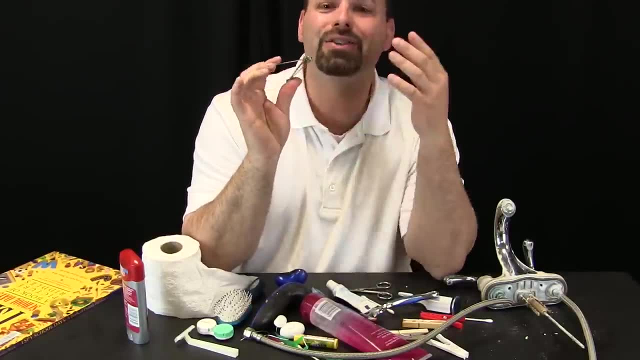 but think about this: Do we see more than one simple machine at work in this fingernail clipper? I see the wedge up front, but what am I doing here with this part of the fingernail clipper? I think it is a lever. I have a lever and a wedge. Let us look at our scissors. 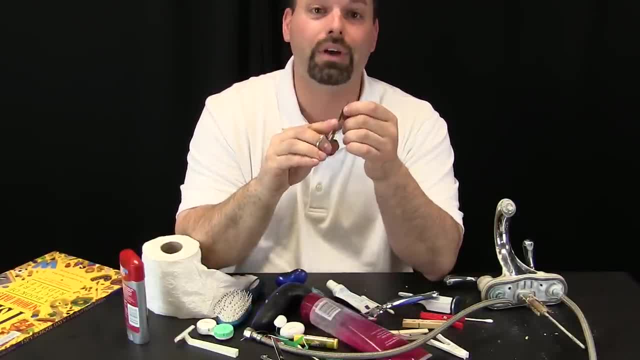 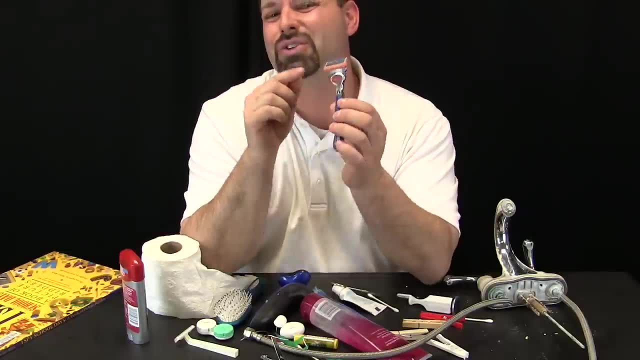 Can I cut and clip with this? I will try my fingernail again, or maybe I will cut a part of my beard, I do not know. trim it up. I think it does cut and clip. And then my razor. we are going to zoom in so you can take a closer look at the blades on this razor and you will see. 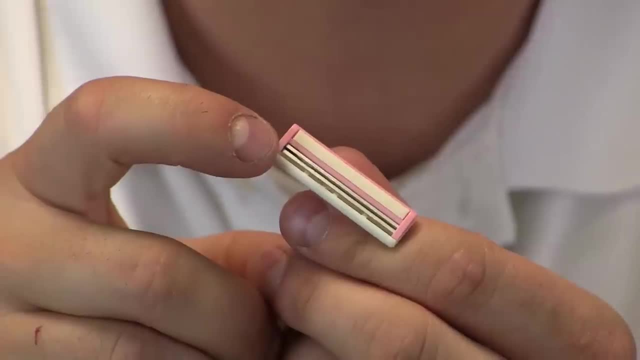 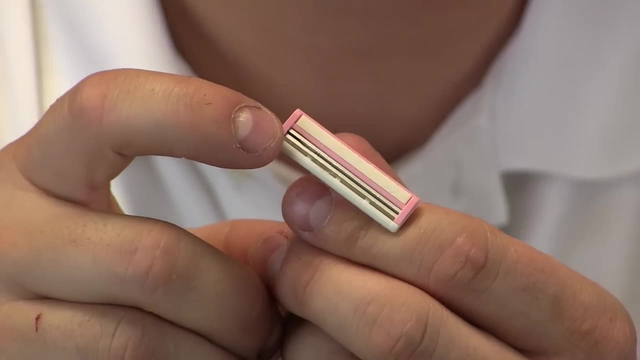 that they do cut and clip. We have zoomed in so you could see the blades on this razor, and those blades are actually wedges that separate, cut and clip hair that I could shave my face. And now we are ready for the last line of our poem. I try some wheels and axles that spin. 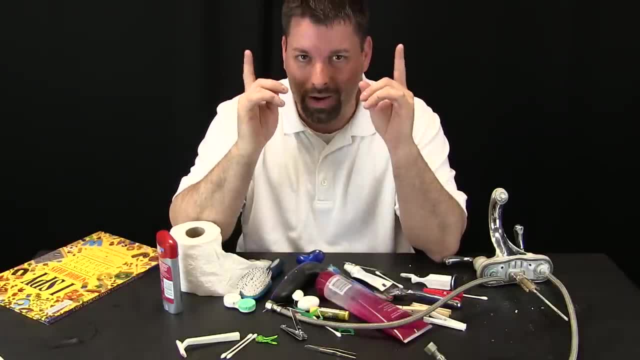 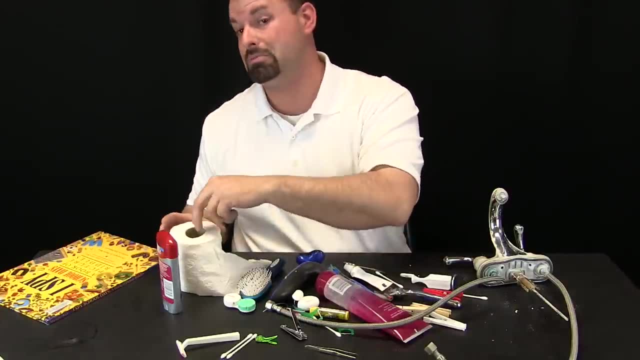 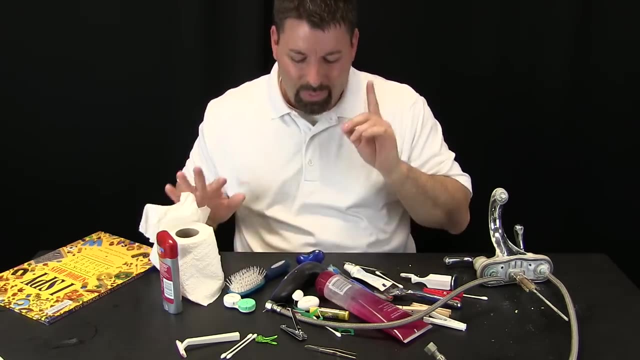 what simple machine is a clothespin? All right, here we go. Wheels and axles that spin. Well, I think I see two things that spin. One is obvious: Good old toilet paper. but the other one is not so obvious. I have a container of floss. Now watch. 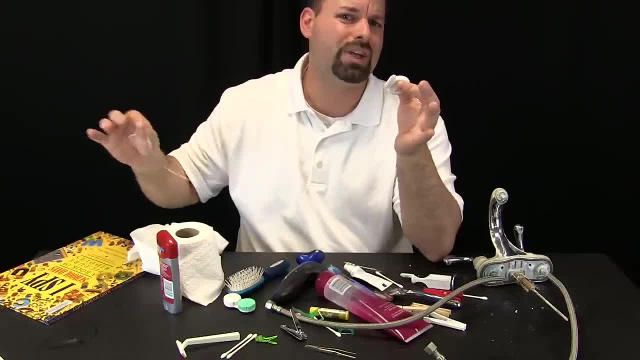 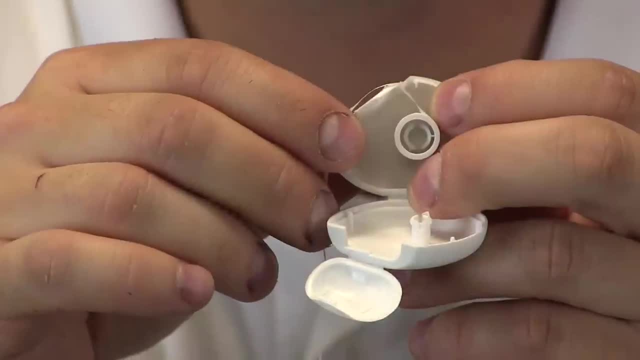 what happens when I pull this string: It comes out. So what is going on inside this container of floss? Let us take a closer look by opening it up. We have opened up our container of floss and zoomed in so you can see the wheel and axle in the center And watch what happens when I pull. 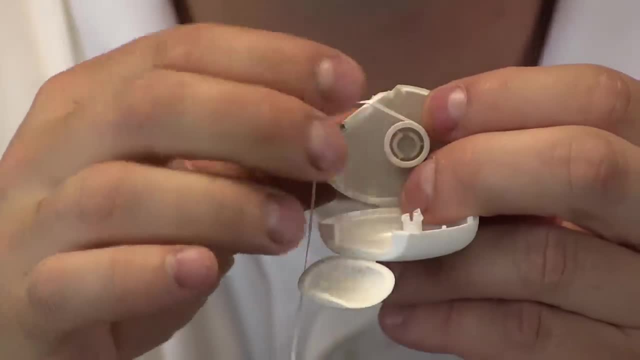 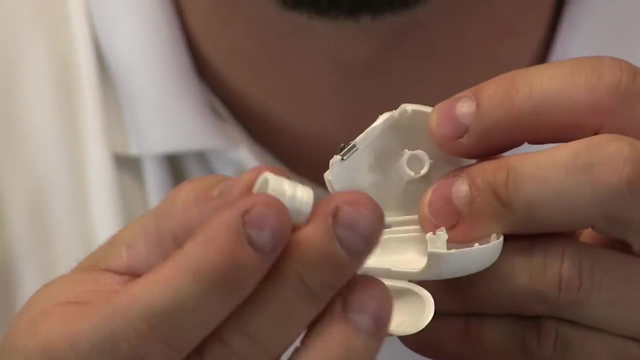 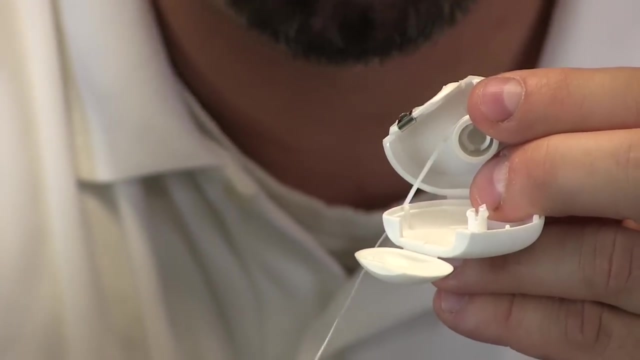 my string of floss. It spins. I try a wheel and axle that spins. It actually wants to come apart. I might be able to. I can pull it out and you can see this slides over the axle and it spins. Cool. 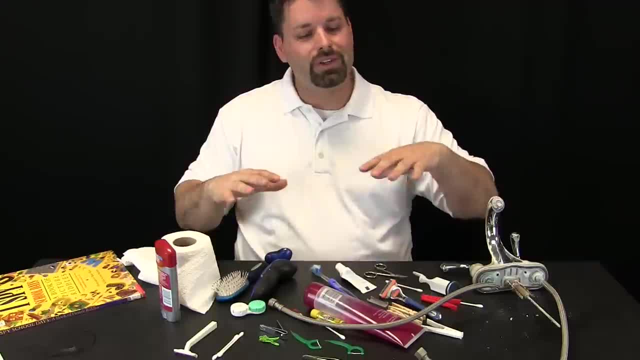 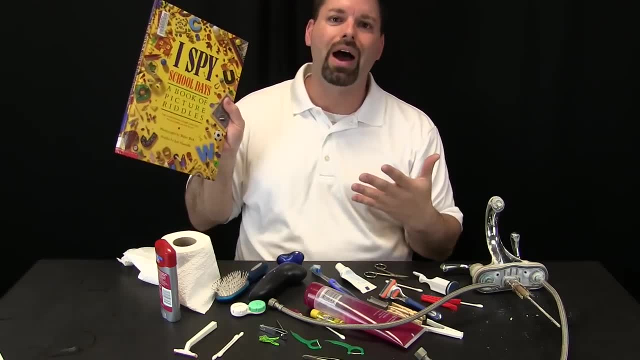 There is a lot of answer to this question. It is a really simple machine that you cannot measure to even understand. Is this a tool? Is it not amazing how simple machine science is simply everywhere? We patterned this idea of I try science after the book series I Spy.